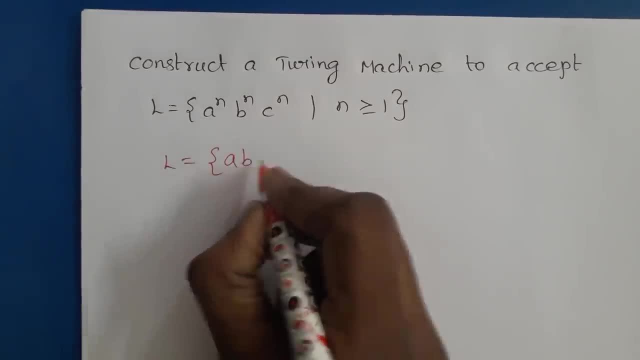 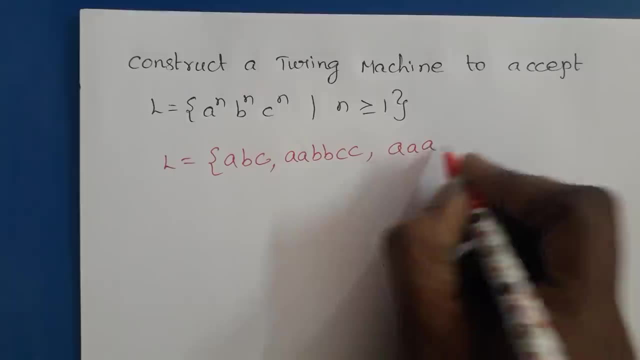 That is, L is equal to a b, c If n is 1, a b c If n is 2, w a, w, b, w, c, triple a, triple b, triple c, and so on. 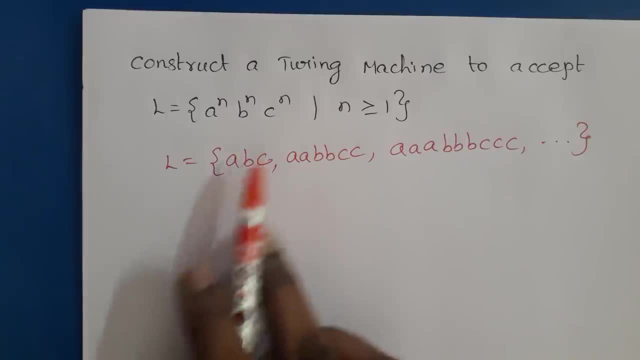 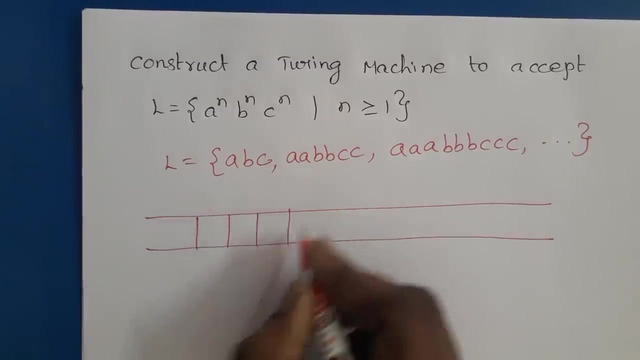 So our Turing machine has to accept the following: these input strings. Other input strings must be rejected by our Turing machine. So initially we need to load the input string on the tape. Turing machine has an infinite tape as a memory, So it is infinite to both the left and right end. So the tape is divided into cells. Initially we need to load the input string on the tape. 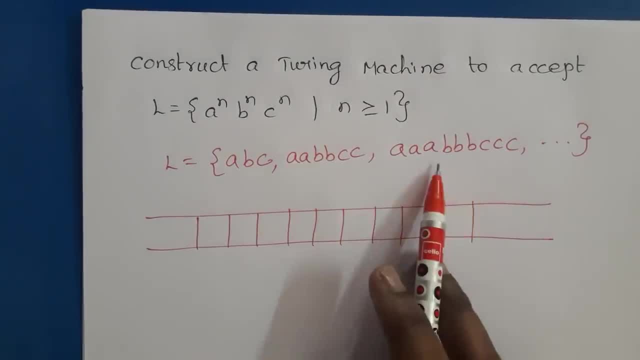 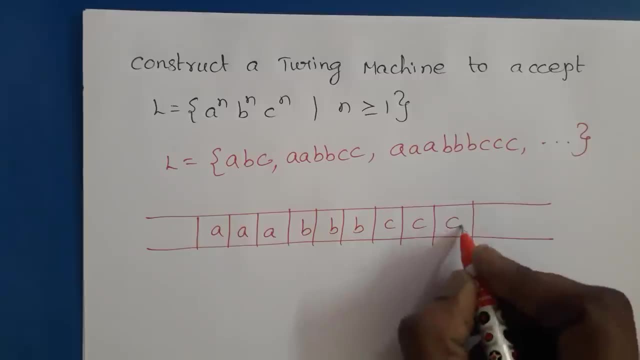 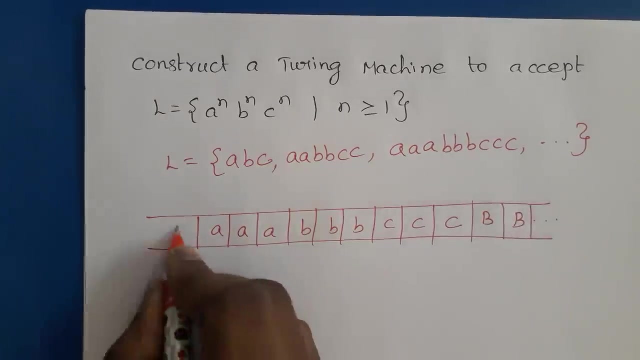 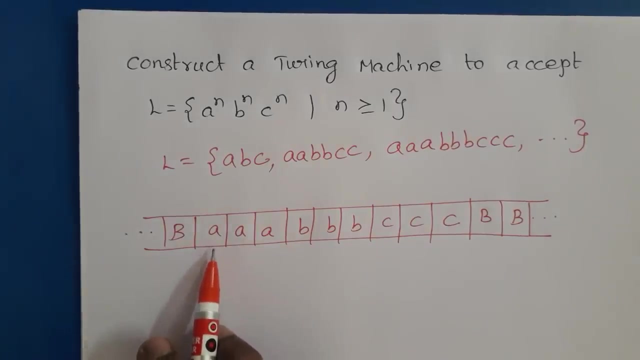 So I am going to take this string as an example. So a, a, a, b, b, b, c, c, c must be loaded on the tape. The remaining cells will hold blank. Initially, the read write head will scan the first symbol of the input string. So initially it is scanning the a first, a. 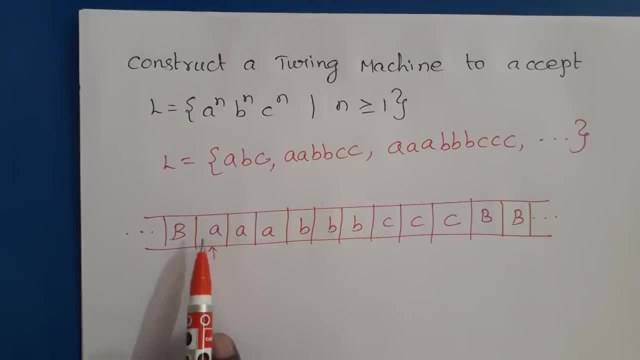 The idea here is we need to match first a with first b and c. So for that matching process we are going to use three symbols: x, y and z. So a must be replaced by x. So a must be replaced by x. So a must be replaced by x. 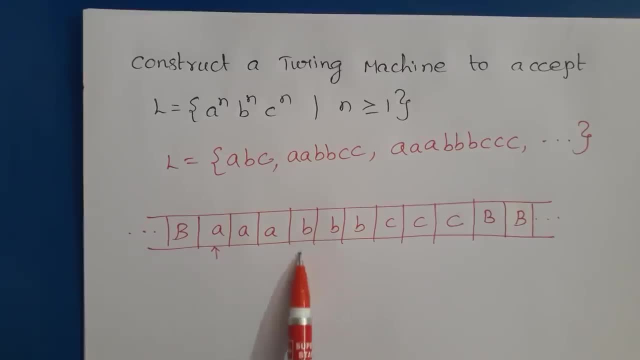 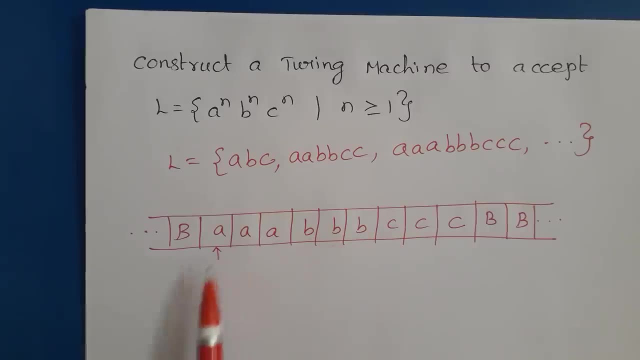 After matching a, b c, we need to move forward. Then b must be replaced by y, Then c should be replaced by z. After matching a, b c, we need to move left until we have seen x, Then again, second a, b, c must be replaced. 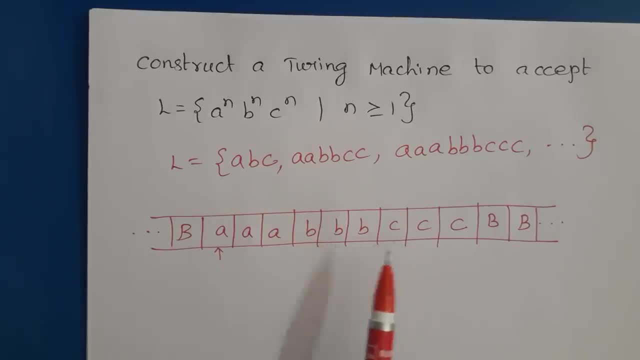 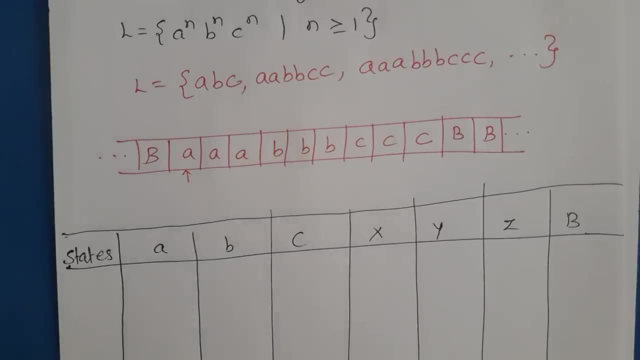 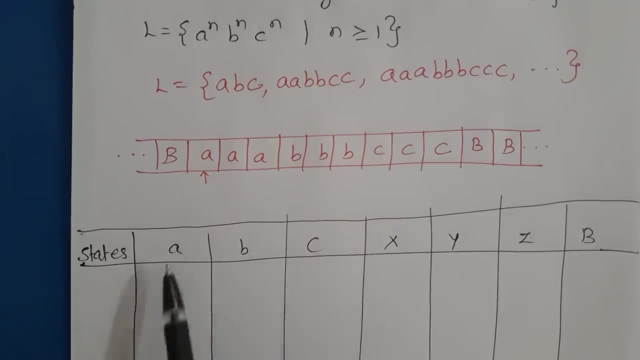 So this is the idea. So first we need to construct the Turing machine table for that, The Turing machine table, In which rows correspond to states and columns correspond to the tape symbols. Here the tape symbols are a, b, c, x, y, z and blank. 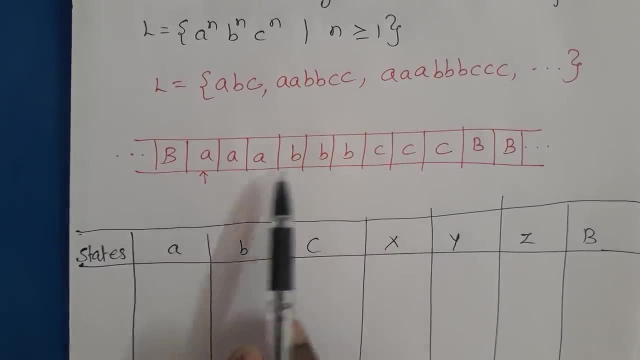 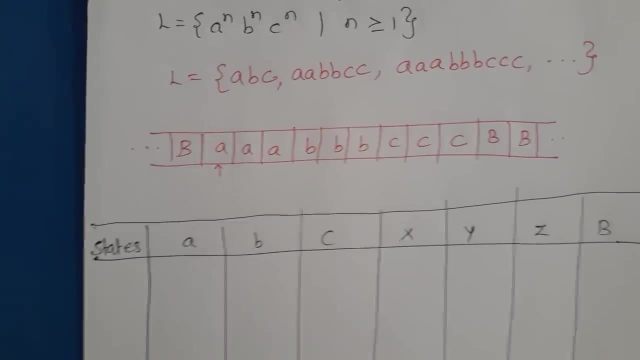 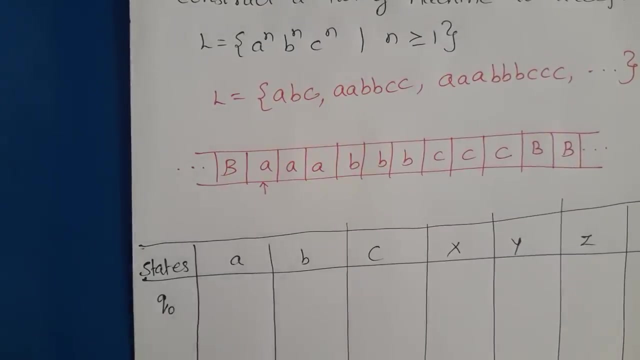 These a, b, c, a's, b's and c's are replaced by x, y and z, then blank. So these seven symbols are columns and states are the rows. So initially our Turing machine is in state q0.. And first the read-write head is scanning a. 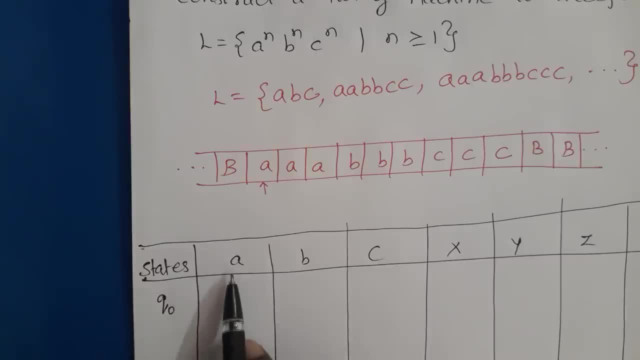 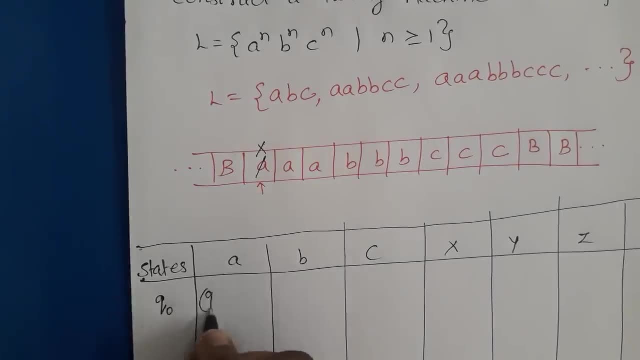 So if the Turing machine is in state q0 and the tape symbol is a, then this a must be replaced by x And the state should be changed to q1.. So q1, a is replaced by x and movement of the tape head is right side. 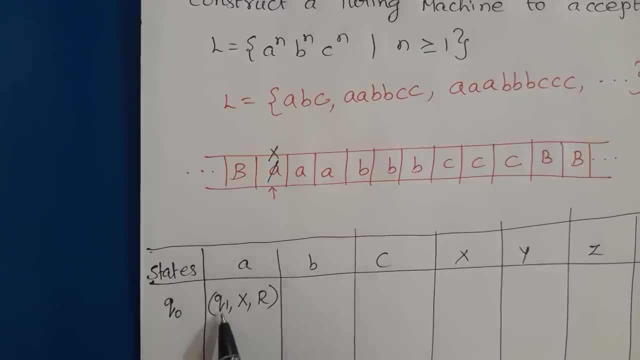 So right Here we need to change the state, Otherwise all a's will be replaced by x. If you search Q0 here, then this will become the infinite loop, now loop. So all a's will be replaced by x. But we are going to match one a with one b, then with one c. 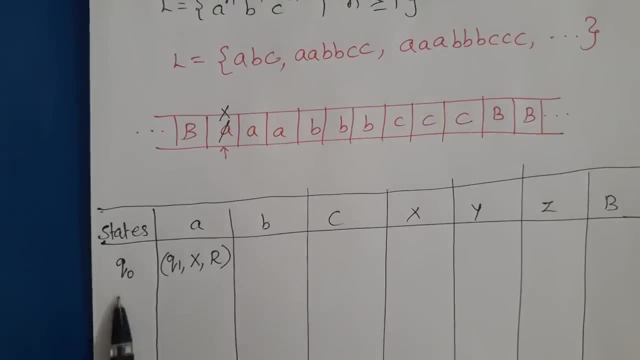 So state should be changed to q1 and move is right side. A is replaced by x. Now the Turing machine is in tape 1 and it is scanning a. So now we need to, we are going to replace b by x for. so for the number of a's, we just move the tape head to the right side. 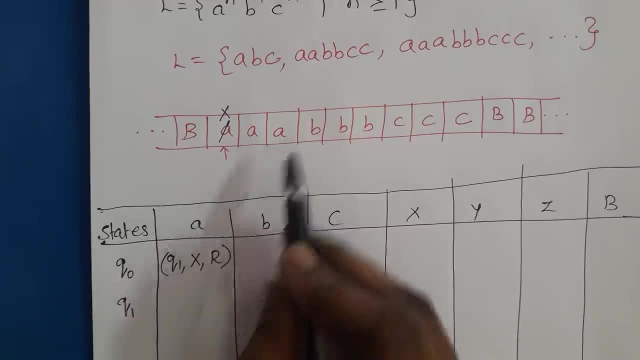 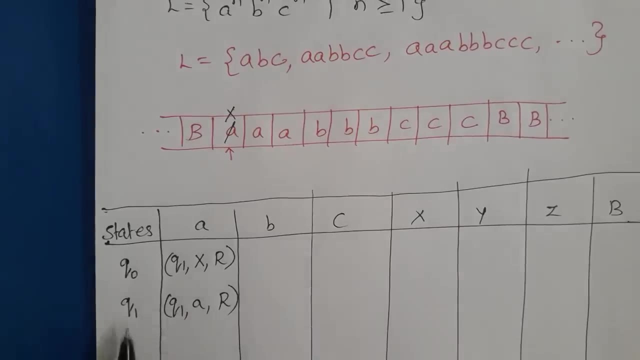 So for the number of a's, it just keep on moving to right, right, right. So q1 comma: a- no change in state and tape symbol: just move is right move, No change in state and tape symbol: a just move is right move. 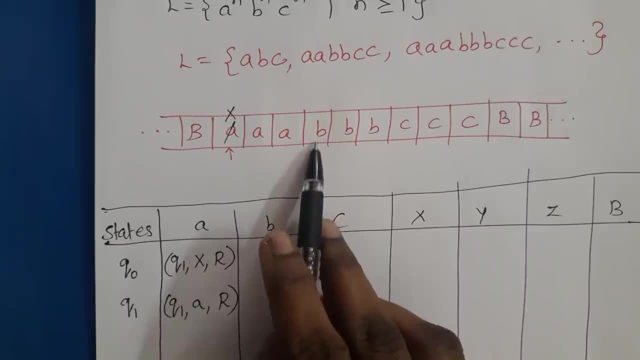 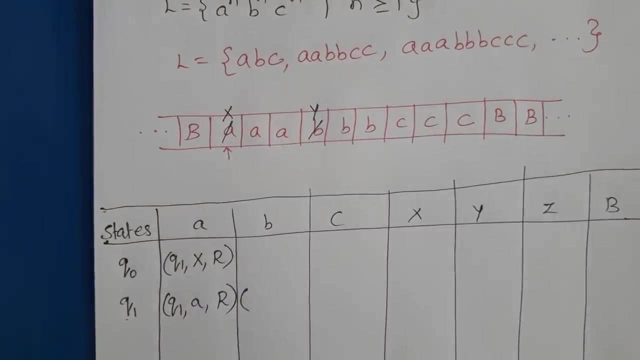 So this is repeatedly performed. Now we are going to see blank in the tape. So in q1, sorry, not blank b in the tape. So in q1, if b is the tape symbol, then we need to replace it by y. 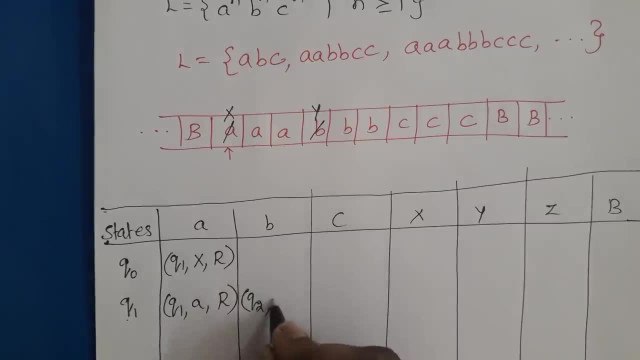 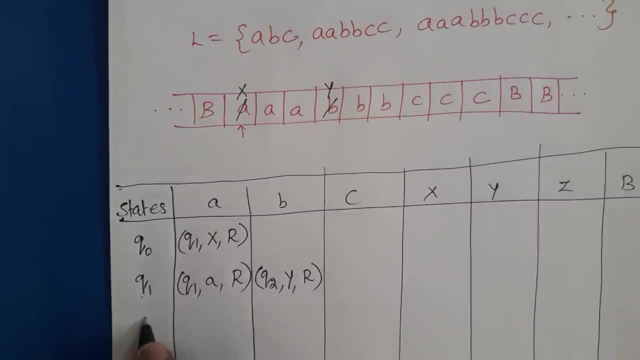 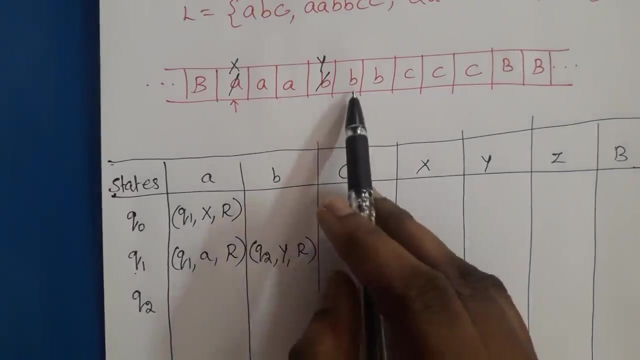 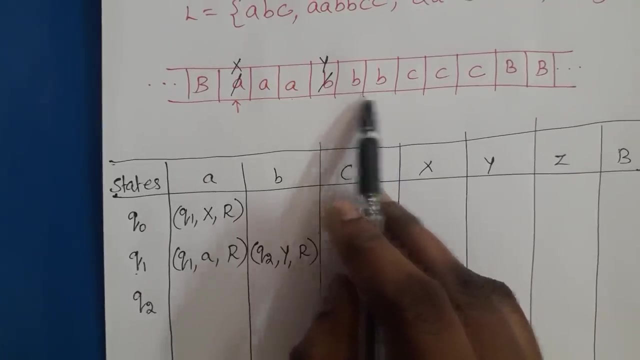 So q1 is changed to q2.. B is replaced by y and the move is right. move Now the tape. the Turing machine is in state q2 and it is scanning b. So now for the number of b's. we just move on to right side until we have seen c. 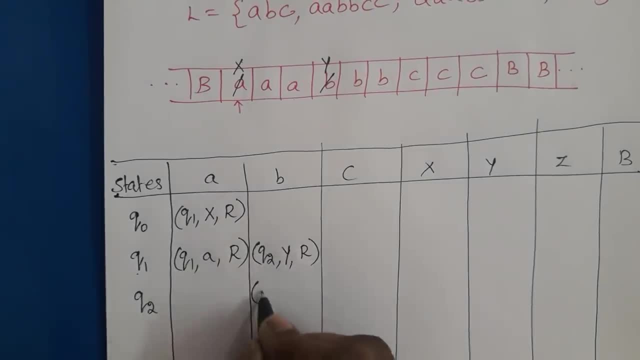 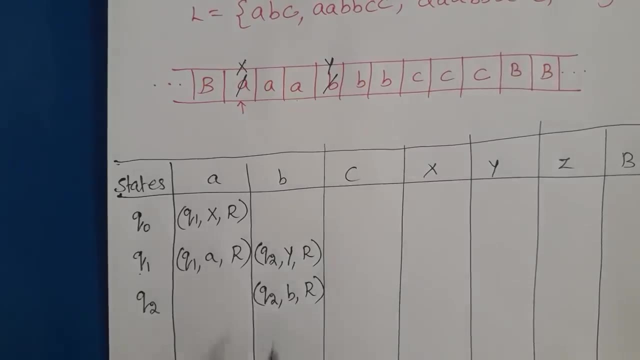 So in q2, if b is the tape symbol, then q2 remains q2, b remains b, move is right move. So, after recognizing all b's, after scanning all b's, we will scan c at one point of time. 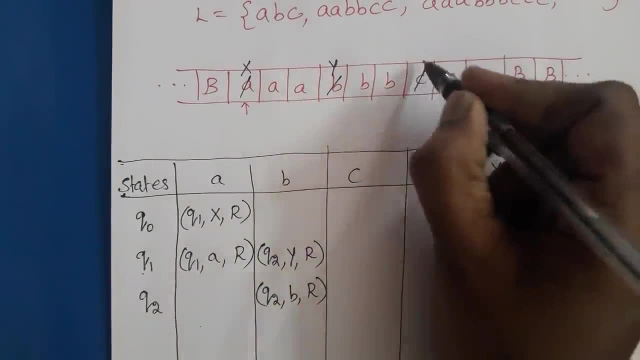 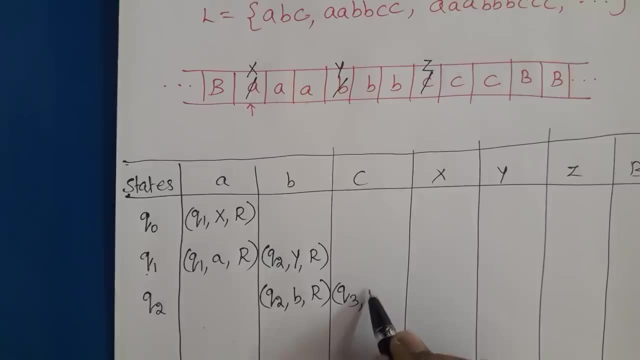 So in q2, if c is the tape symbol it should be replaced by z. So in q2,, if c is the tape symbol, state should be changed to q3.. C is replaced by z and then move is left move. 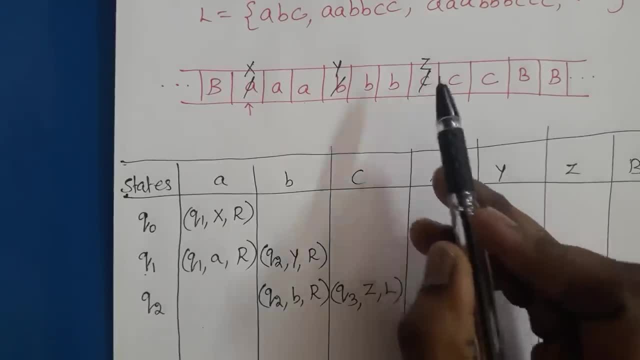 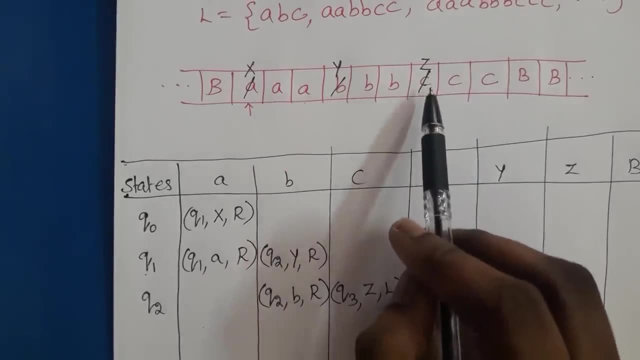 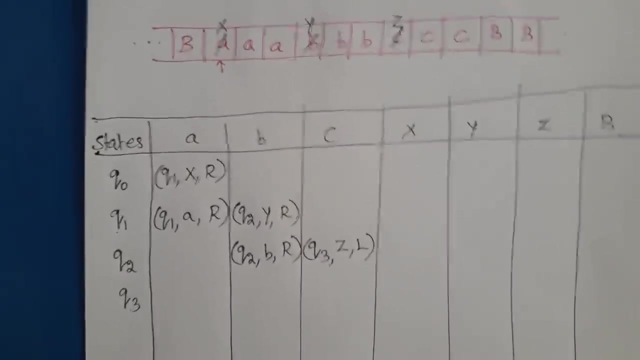 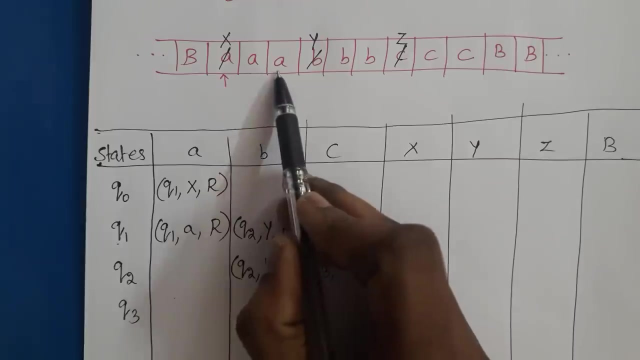 Because after replacing the c by z we need to match the second cycle, that is, second a, b and c. So we need to move the tape head to left side. So now the Turing machine is in state q3.. So here for the number of b's, y and number of a's. 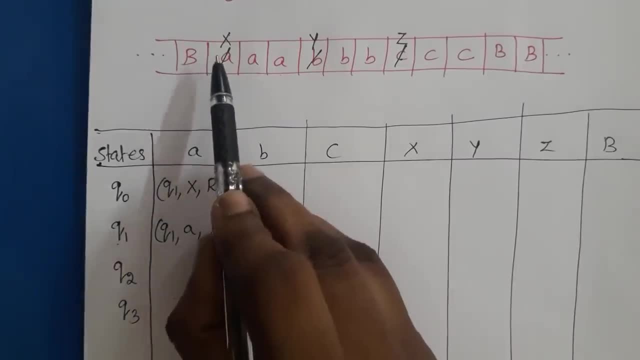 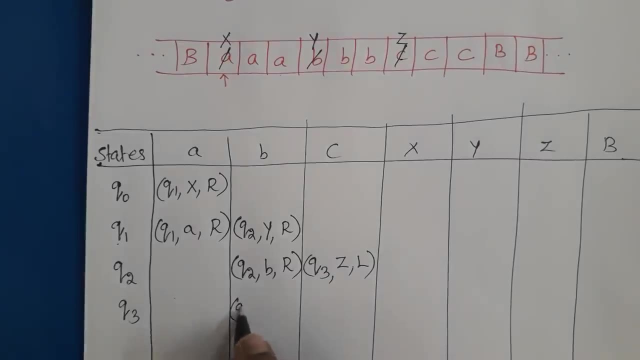 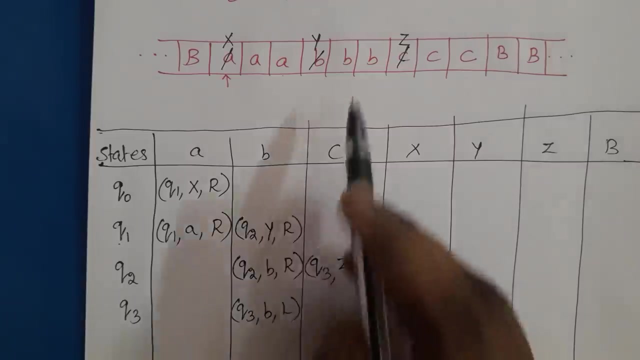 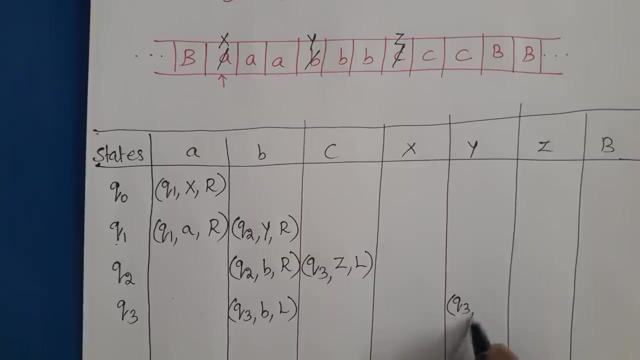 we just keep on, move on to left until we have seen x, So in state q3, if the symbols are b, then no need to change the state and tape symbol, just movement of the tape head is left. Then for y, also in q3, if y is the tape symbol, then q3 remains q3. 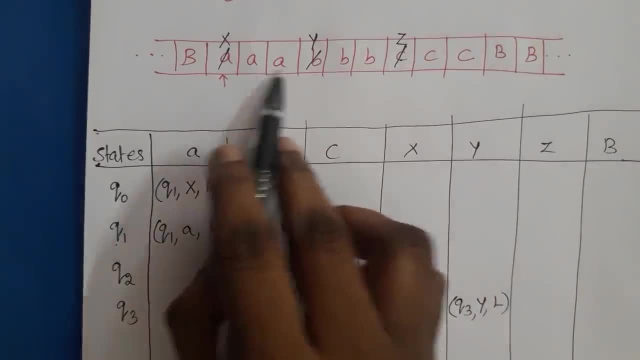 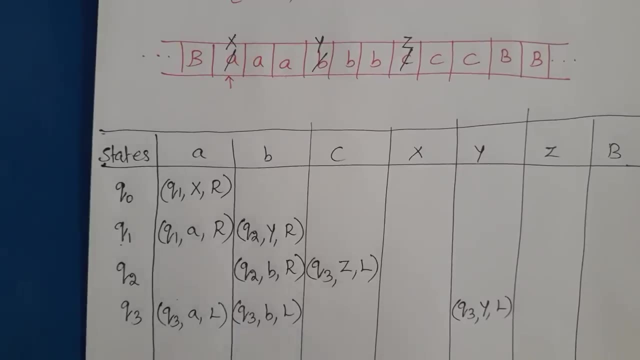 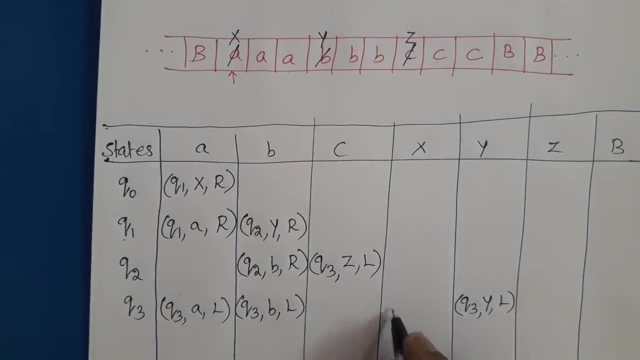 Tape symbol is y move is left, Then we will see number of a's, So q3,. a move is left move, Then we will see x next time. So in q3, if x is the tape symbol, then state should be changed to q0. 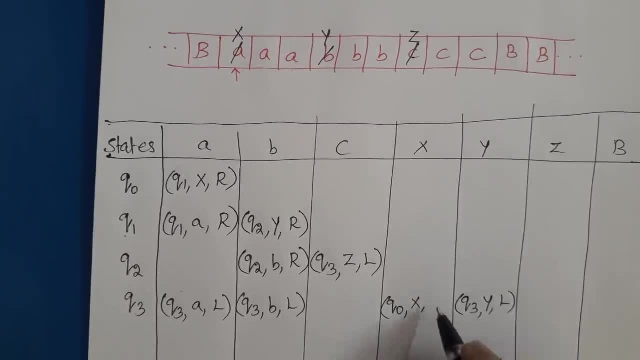 So x remains x and movement of the tape head is right side. Here the state should be changed to q0, because in q0, next cycle begins, that is, we are going to match a, a, b and c. So state should be changed to q0. 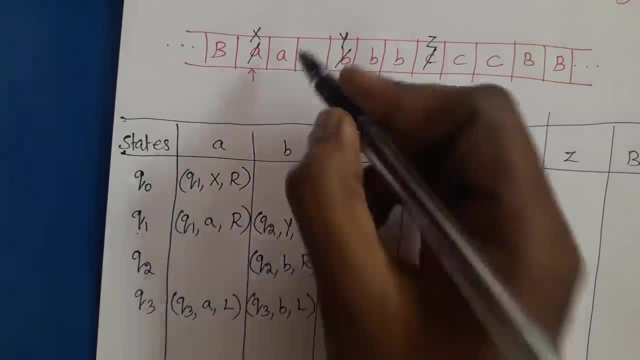 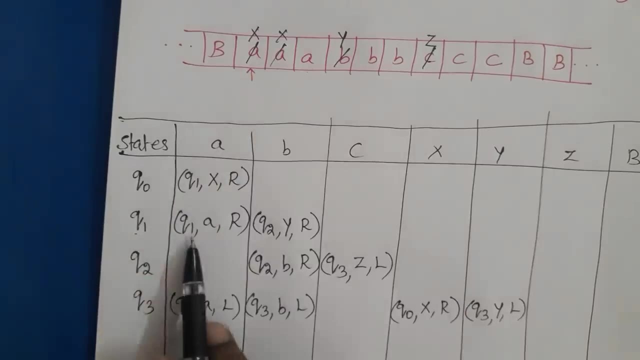 So now in q0, if a is a tape symbol, it is replaced by x and state changed to q1,. move is right move. So in q1, for number of a's, simply it moves the tape head to right side. 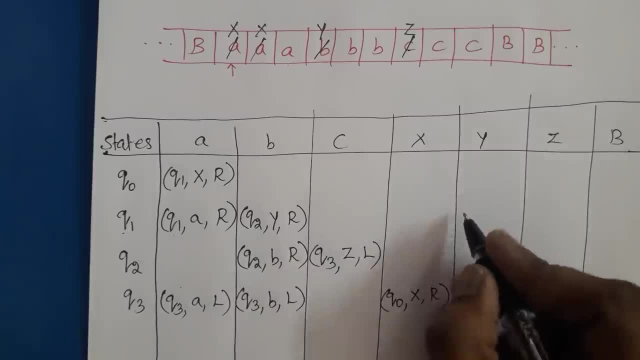 Now it can see number of y's also. So we need to write a transition function for the tape symbol y in state q1.. So in state q1, if y is the tape symbol, then no need to change the state and tape symbol. just movement is right. 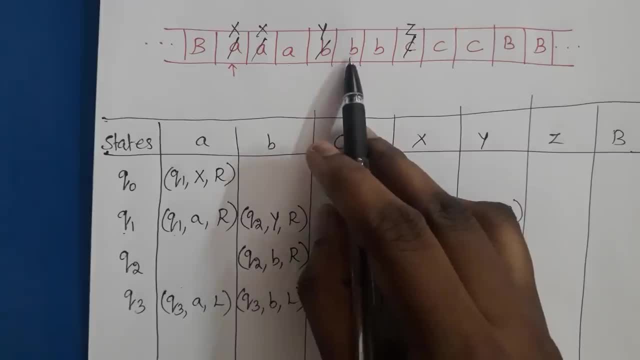 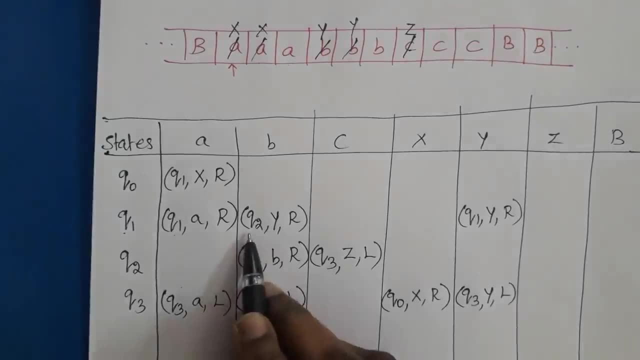 Move is right. move, So we will see b. So now in q1, b is a tape symbol. It is replaced by y and state changed to q2,. move is right. move In q2, for the number of b's, it just keep on, move on to right. 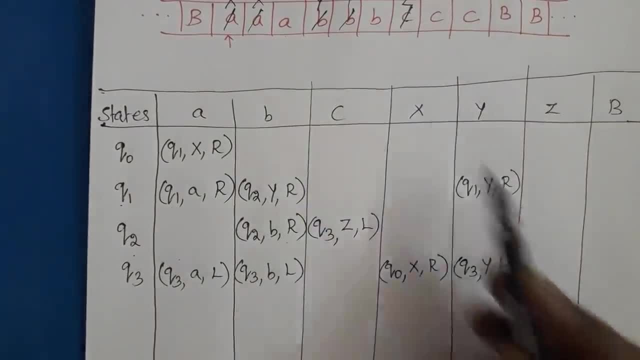 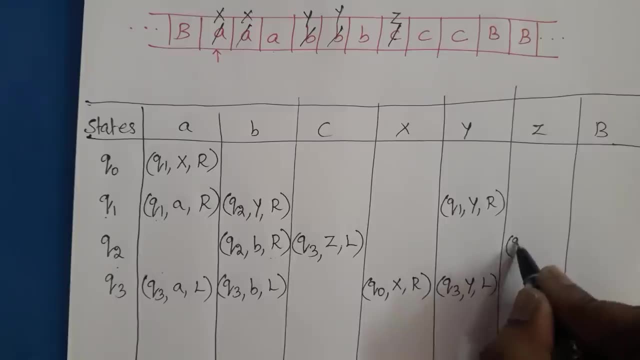 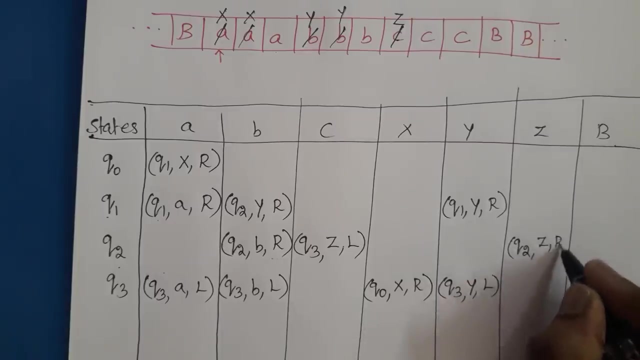 So now we need to write the transition for z also, For the z also. we just keep on move on to right. So in q2, if z is a tape symbol, state is q2,, next state is q2, z remains z, move is right. 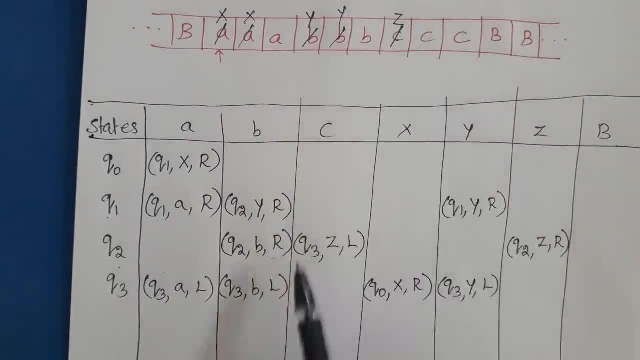 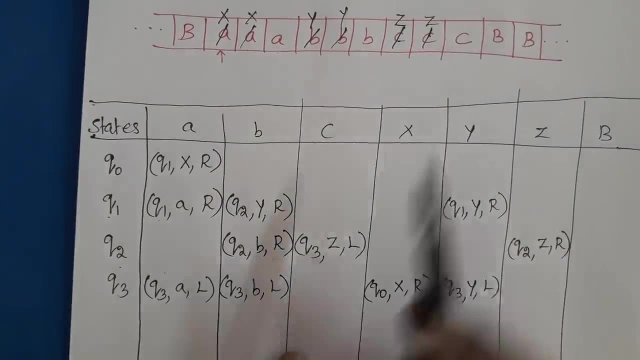 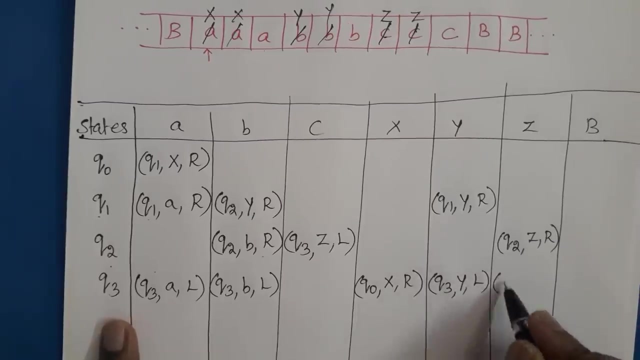 So in q2, now we will see c. So c will be replaced by z, state changed to q3 and the move is left move. So in left move now we will see z also. So in q3, if we will see z, q3 remains q3,. 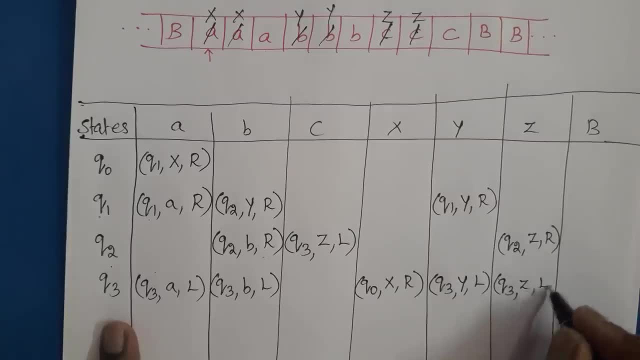 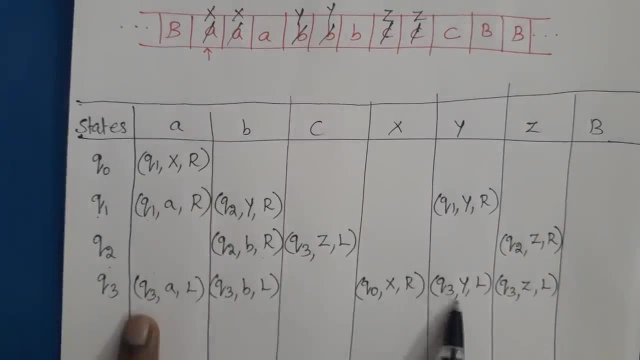 z is not replaced by anything. z remains, z move is left move Now for the number of b. the tape head will move on to left. For the number of y's also, it is going to move on left. Then for number of a's left. 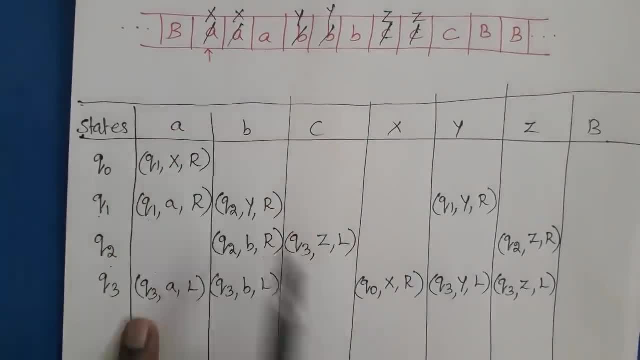 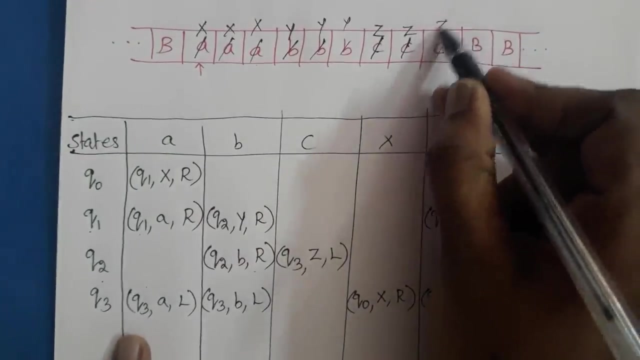 So this is repeated until we have seen x. Whenever we see x, the state changed to q0 and x remains. x move is right move. So now the same step is repeated, So this a will also be replaced by x, Then this will be replaced by y, and this will be replaced by z. 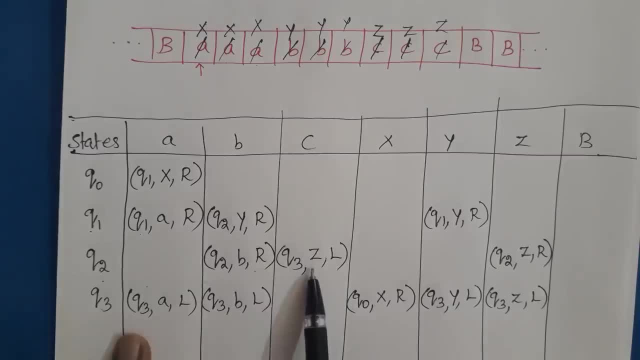 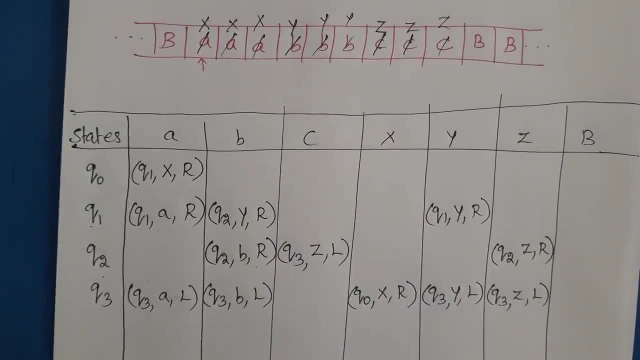 So after replacing this c by z, we will move our tape head. So after replacing c by z, this c by z for the number of z, we will just keep on move on to left, Then for number of y's, then for number of, then for x. 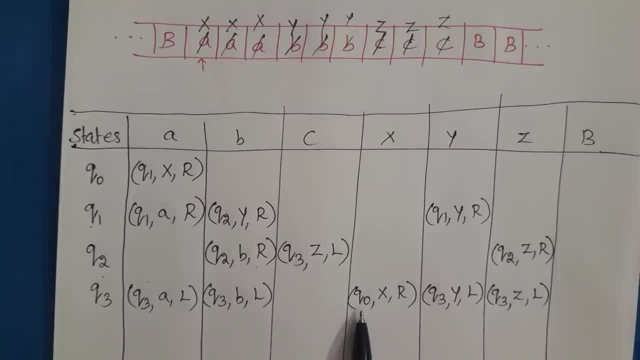 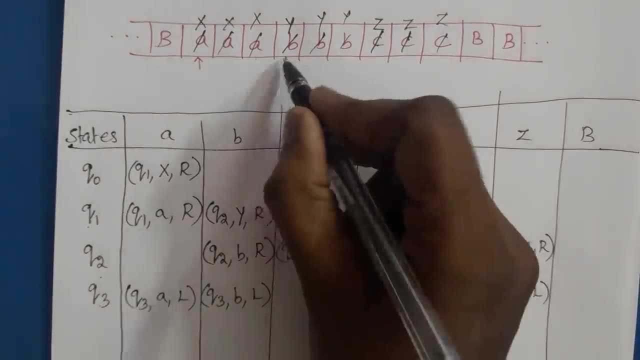 Then for x, our tape head is move on to right side and the state changed to q0.. So in q0, so now the tape head is scanning this symbol. So in q0, if another a is there, then that will be replaced by x. 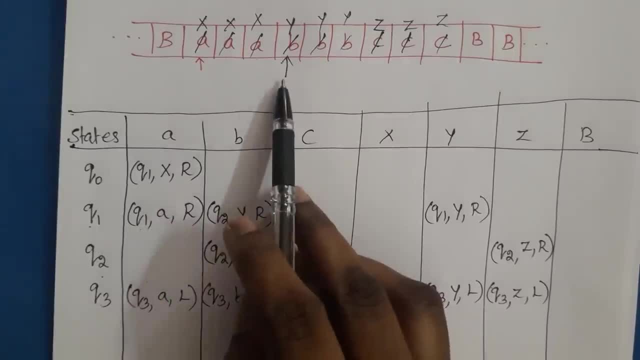 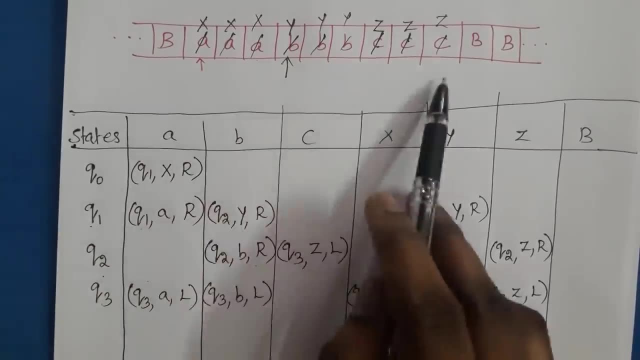 That is, the matching cycle continues. But now the next tape symbol is y. The thing. the meaning is: we have matched a number of a's with b's and c's, So now we need to. we have recognized a number of a's. 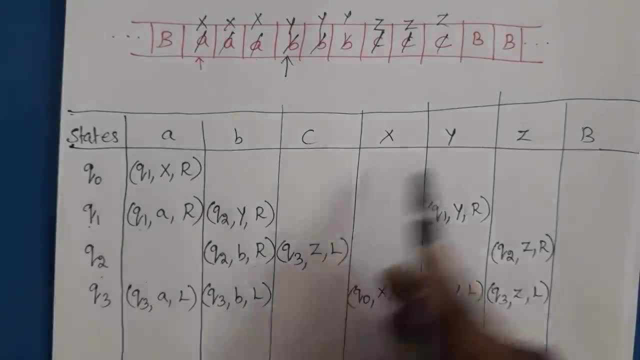 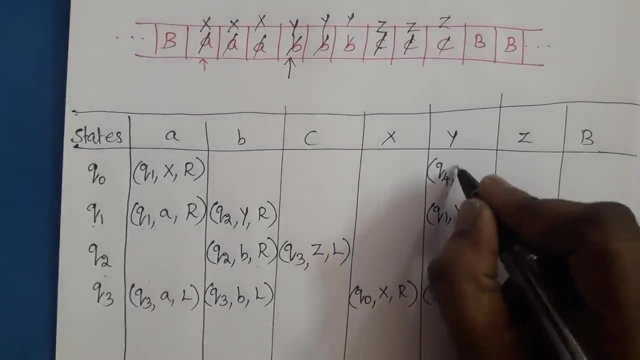 So that should be matched with a number of b's. So in q0,. if y is the tape symbol, then it should be. the state should be changed to q4.. y remains. y move is right move. So in q4,. 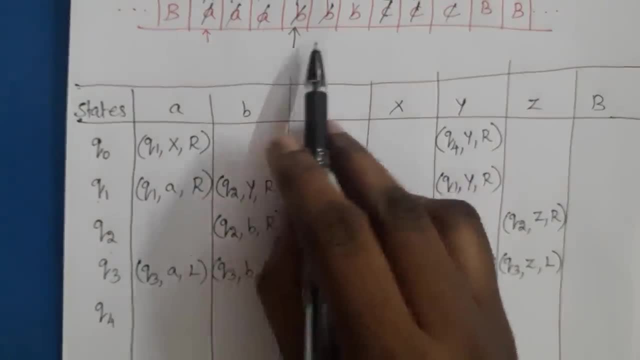 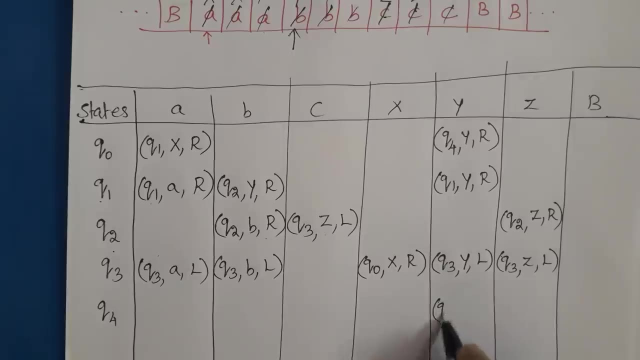 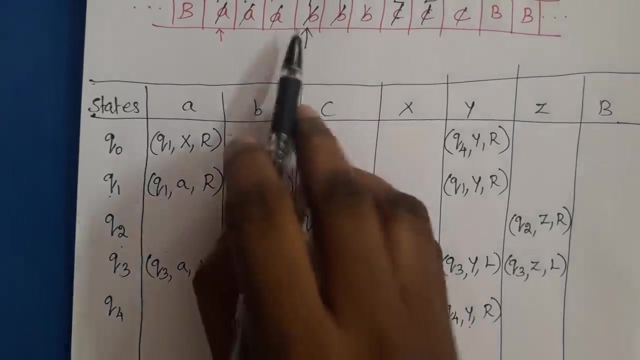 in q4, we will again going to see, going to see some number of y's. So in q4, again, y is the tape symbol, q4 remains q4, move is right move, y remains y. So we just 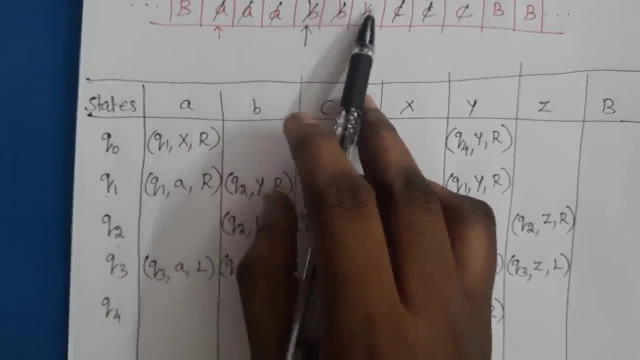 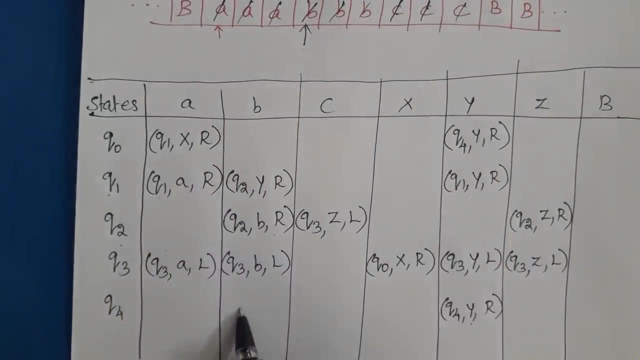 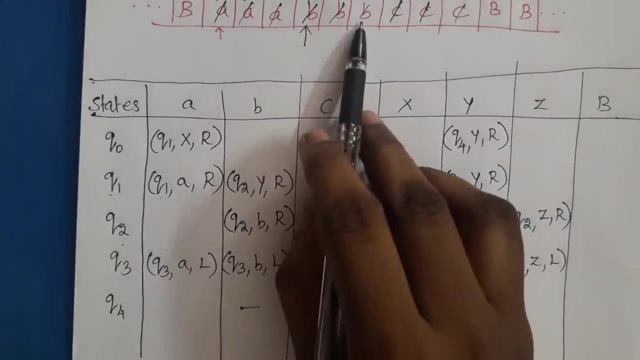 we just keep on moving our tape head to right side. If there is any b is left out, then the input string is wrong. So there is no transition function for b in q4 and b Similarly. next for: after recognizing all v's, after scanning all v's. 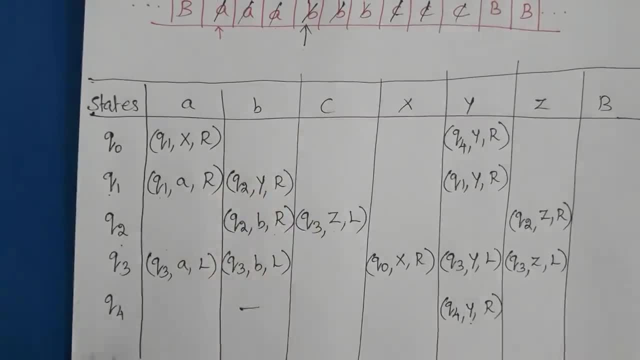 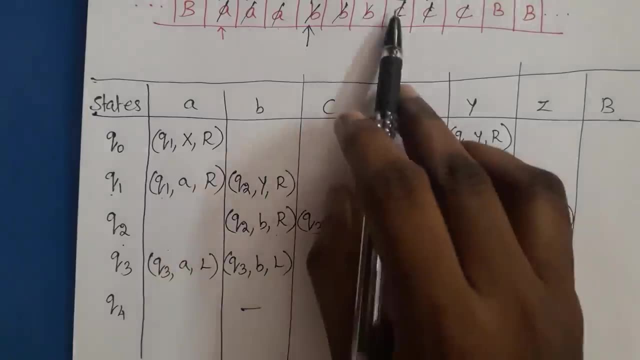 we will. we will start seeing number of z. So in q4, if z is a tape symbol, q4 remains q4, z remains z, move is right move. So after recognizing all c's, all z's, definitely we need to scan blank. 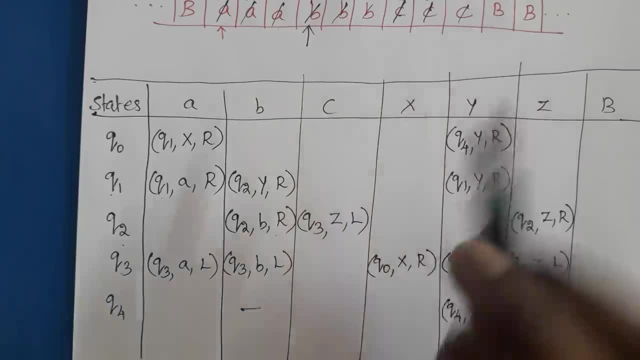 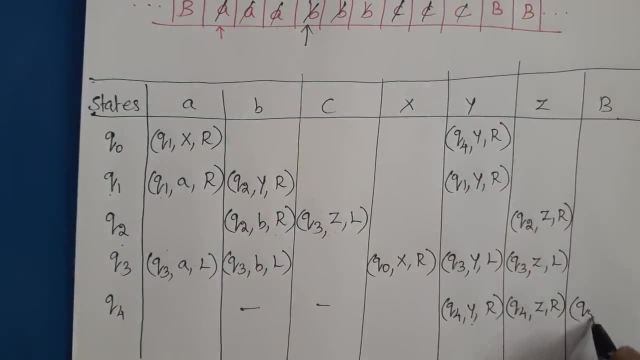 There should not be any c. If there is any c, then the input string is wrong. So there is no transition here. So in q4, if blank is the tape symbol, then state change to the final state. q5,- blank remains blank and the move is right move. 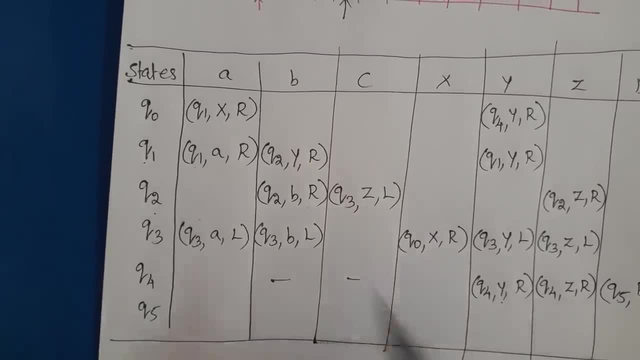 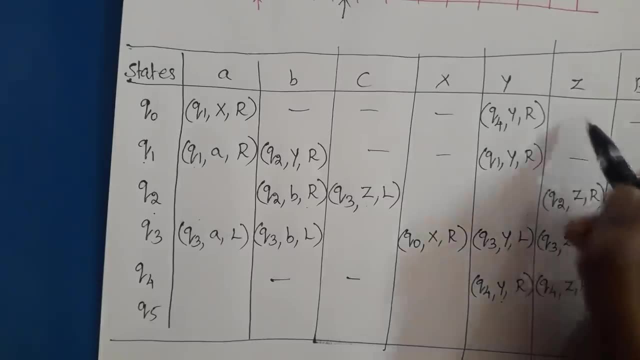 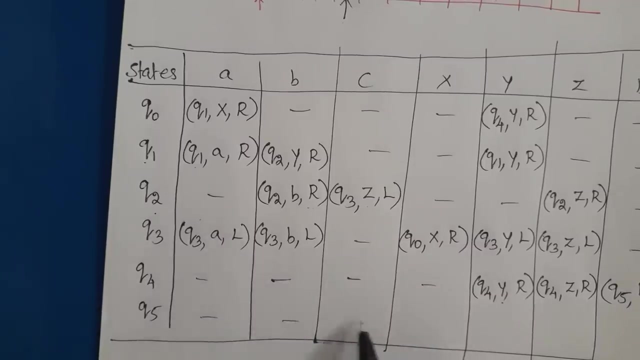 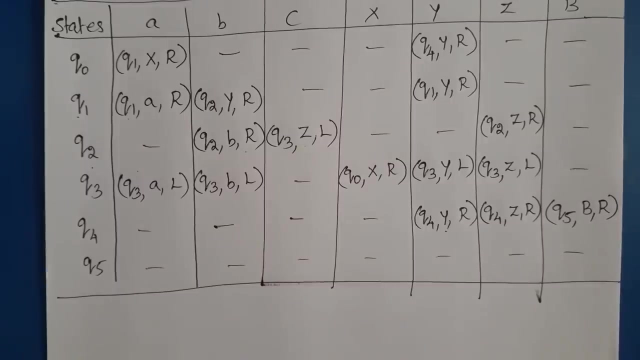 So q5 is a final state. So these are the undefined transition functions. So we need to write the formal representation of the Turing machine. So the Turing machine M has a seven triple notation. First one is set of states. Here the set of states are q0, q2, q5, q0, q1,, q2,, q3,, q4, q5, and set of input symbols. 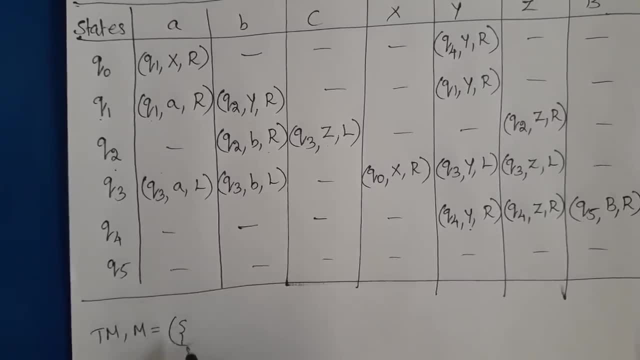 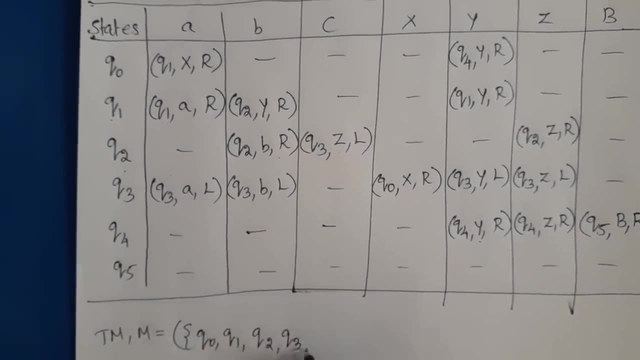 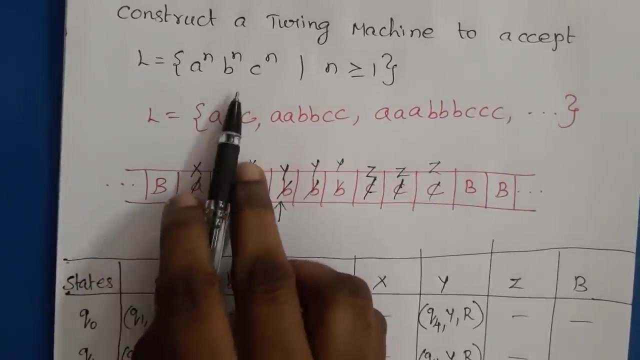 Input symbols are a, b and c. Now we need to write the formal representation of the Turing machine. So the Turing machine M has a seven triple notation. First one is set of states. Here the set of states are q0, q2, q5, q0, q1, q2, q3, q4, q5. 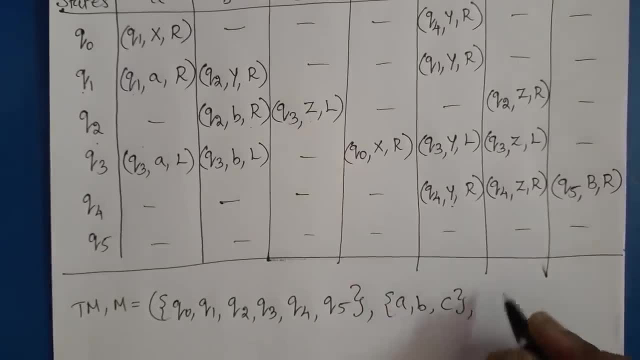 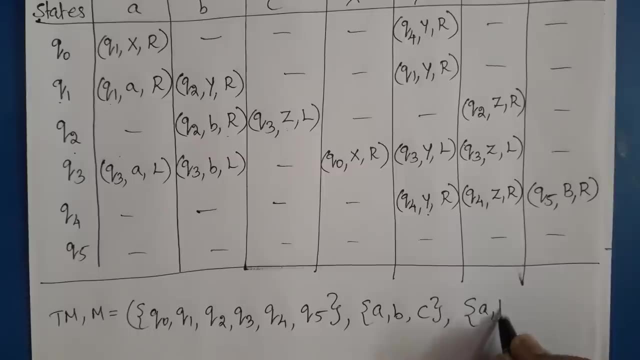 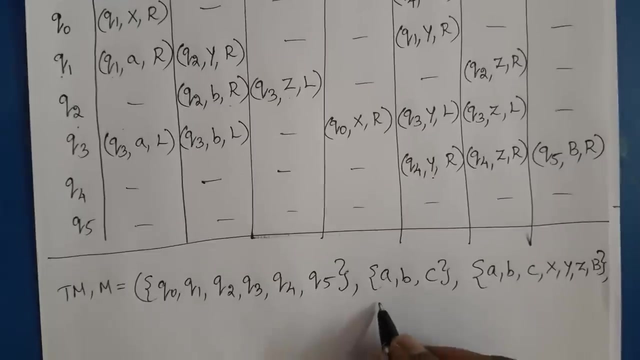 Then set of tape symbols. The tape symbols are: a, b, c, x, y, z and b. a, b, c, x, y, z and b, Then transition function: delta. It is represented as a table. 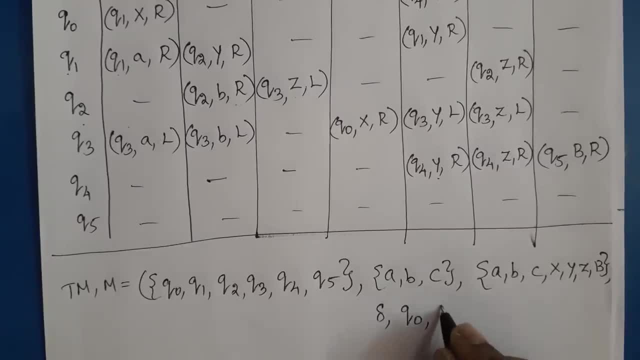 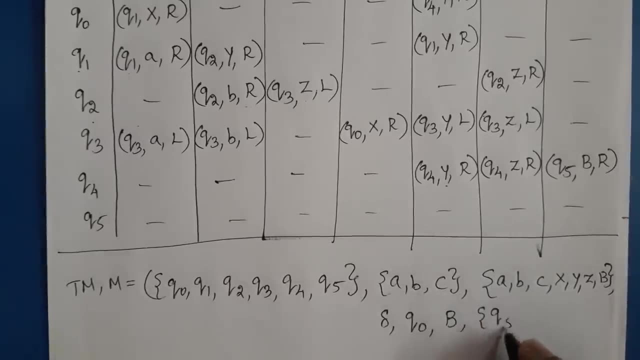 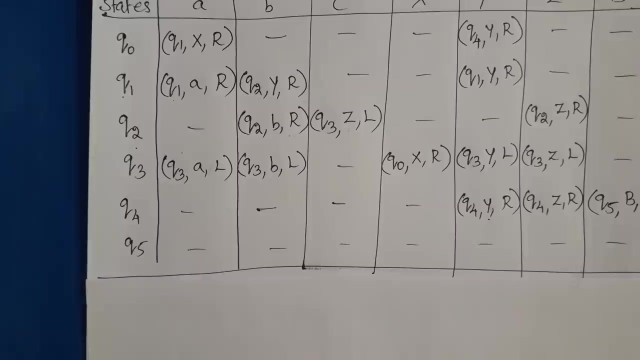 Then start state q0, the special tape symbol, blank, and the set of final states. Here the state is q5.. So q5 is a final state. We can also draw the transition diagram for this problem. Since q0 is a start state, we need to represent q0. 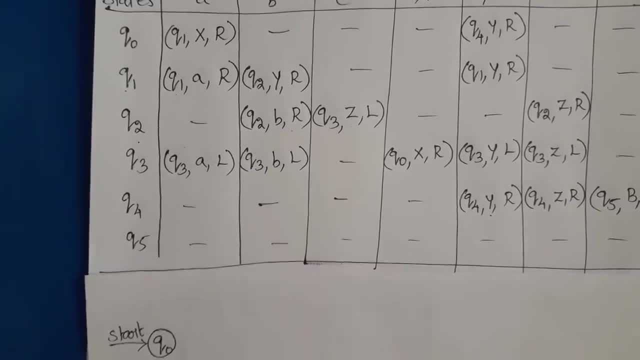 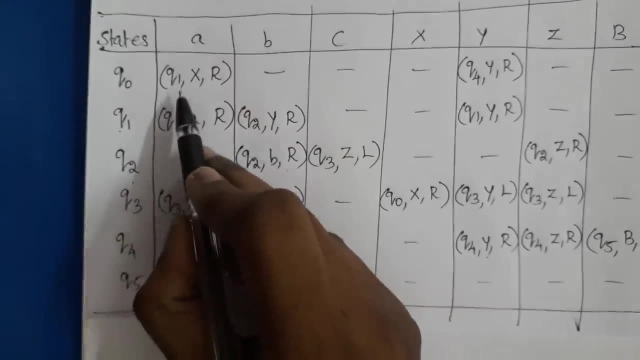 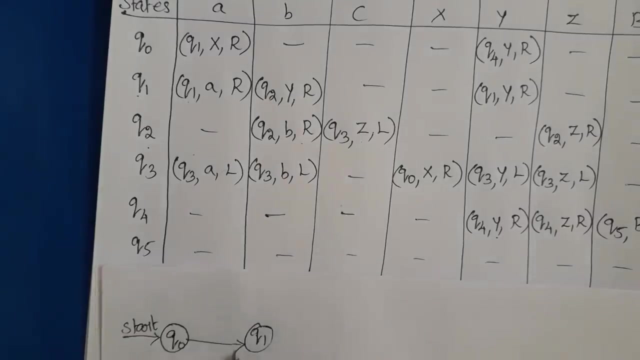 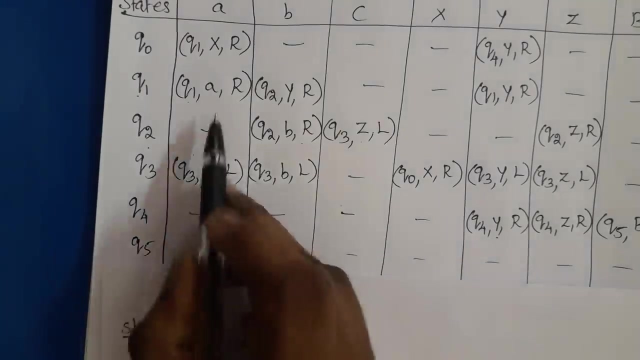 as a start state with an arrow and the label start. Then in state q0, for the state q0 and the tape symbol a state change to q1.. So q1 From q0 to q1, we need to write the tape symbol a forward slash, x, right move x. 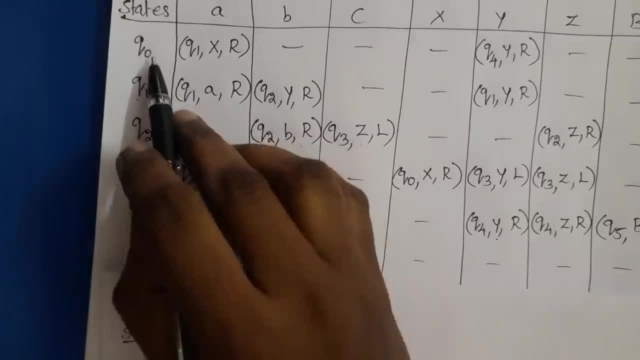 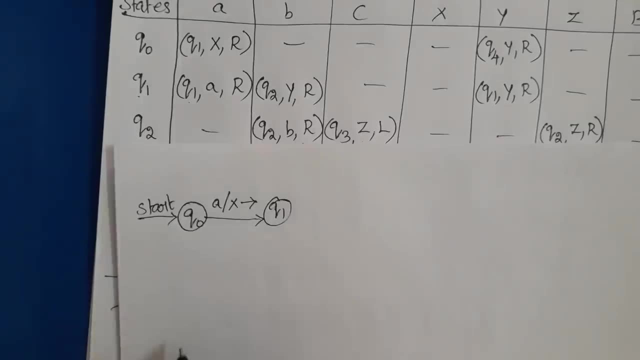 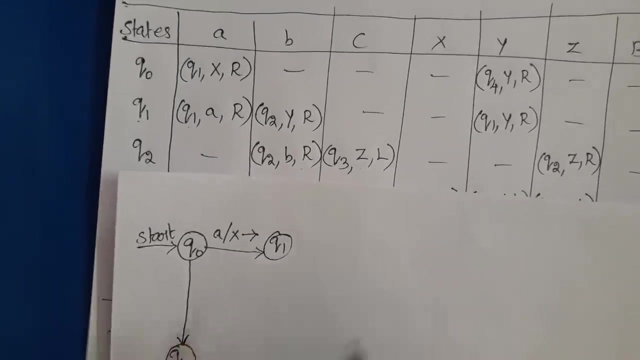 For the right move we need to put right arrow. Then from q0 to q4, we need to draw another transition, So q0 to q4.. The arc is labeled by y slash, y right move, y right arrow. 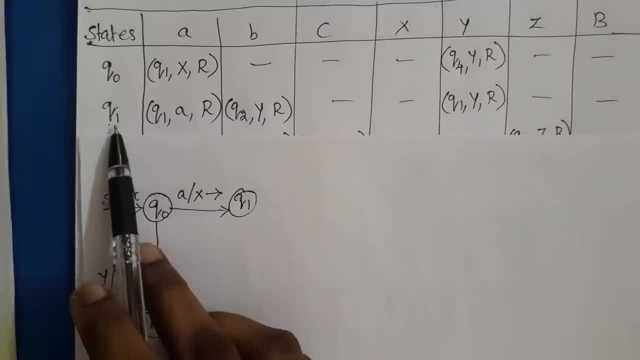 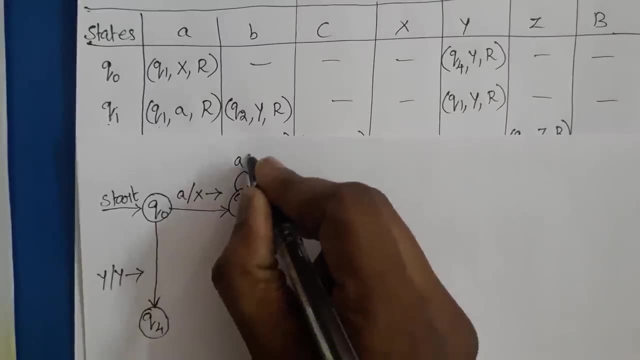 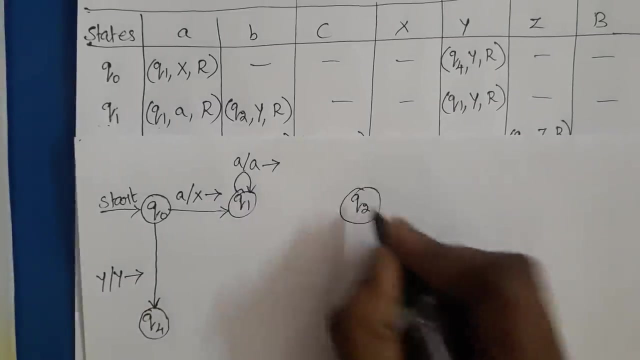 Then, from state q1 to q1, we need to draw a transition That is labeled by a slash- a right move- a slash- a right move. Then, from q1 to q2, the arc is labeled by b slash- y- right move. 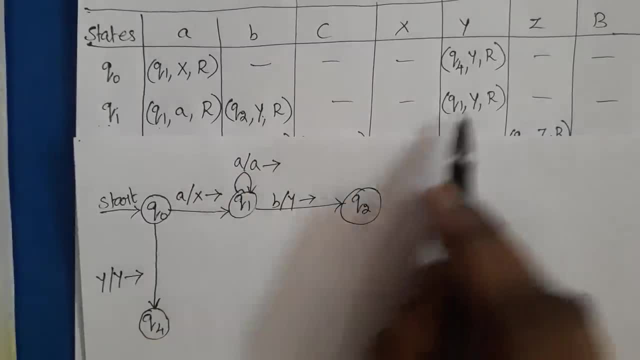 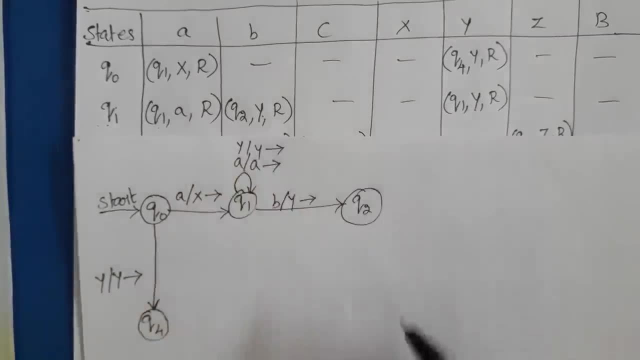 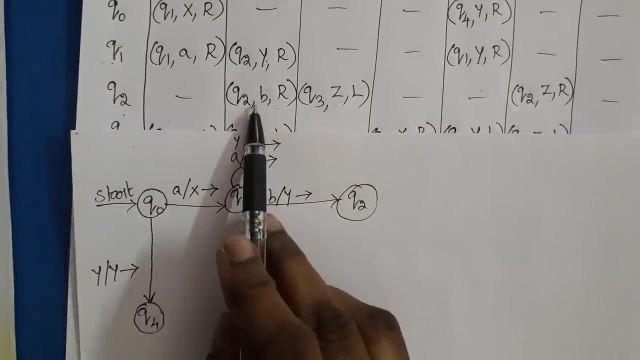 Then from state q1 to q1, another transition is there That is y slash, y right move. Then for the state q2, we need to draw the transition From q2 to q2, there are two transitions. 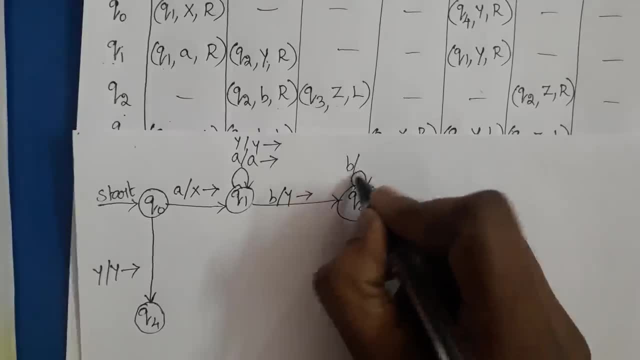 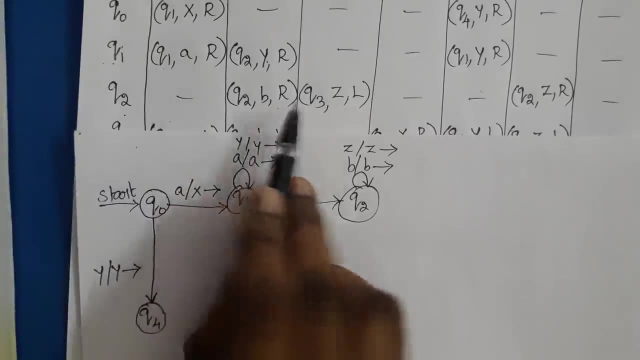 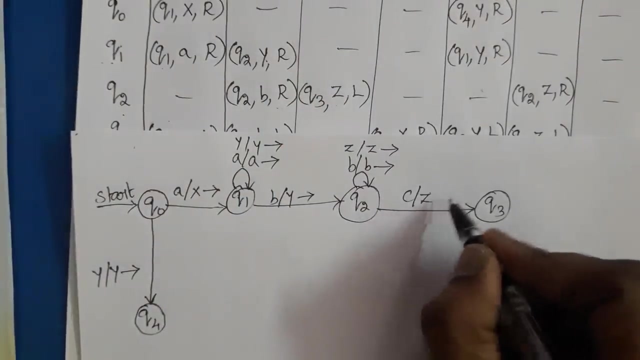 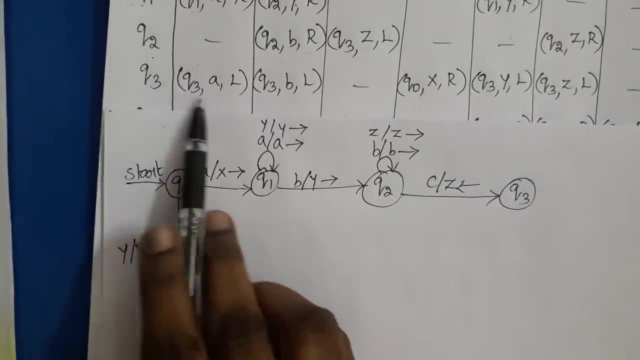 So q2 to q2, b slash b right move, Then z slash z right move. Then from q2 to q3, the arc is labeled by c slash z left move. Then for the q3, from q3 to q3, there are four transitions. 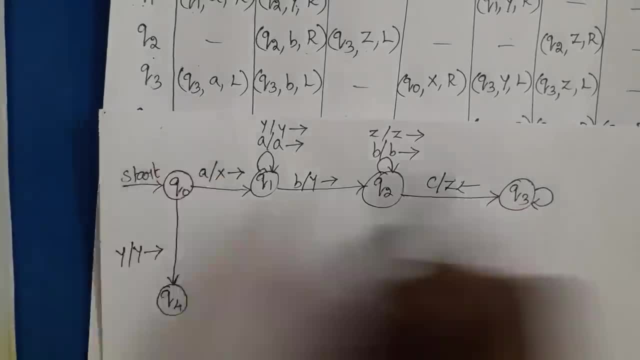 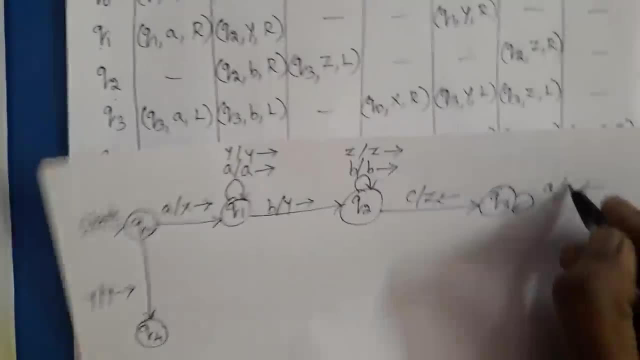 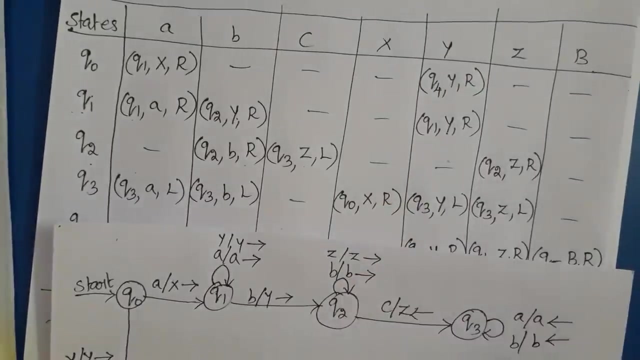 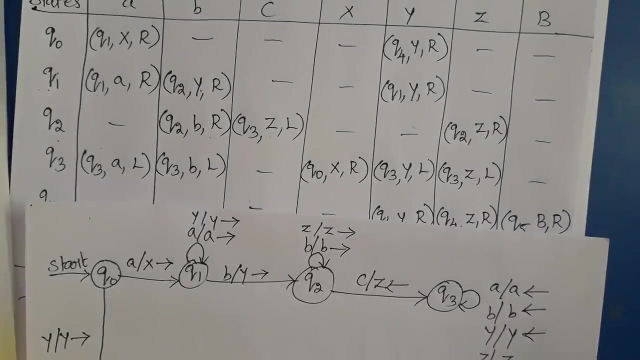 So it should be indicated as a self loop: a slash a left move, Then b slash b left move, Then y slash y left move, Then z slash z left move, Then from q3 to q0, there is a transition. 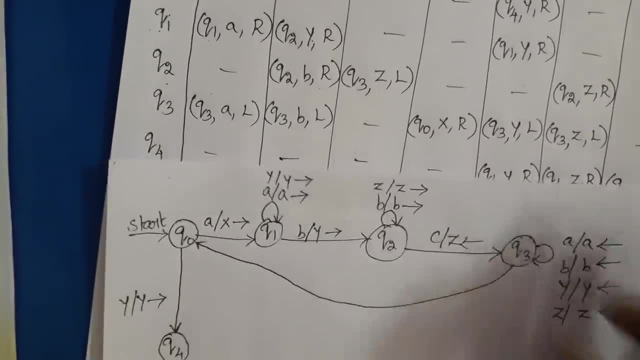 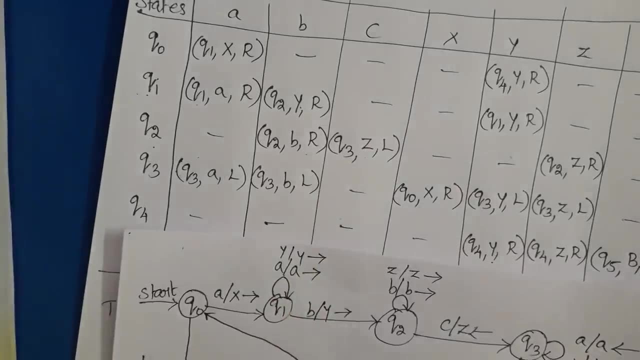 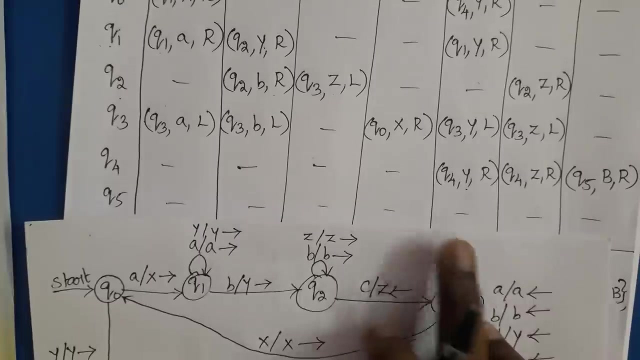 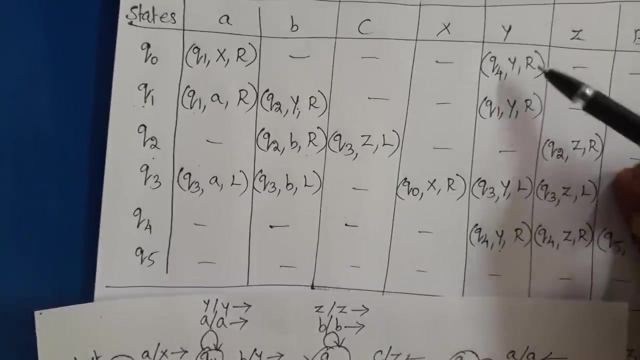 So from q3 to q0, we need to write x given x, x slash x right move. Then for q4, there are three transitions for y. So now q4 to q4, y slash y- right move. 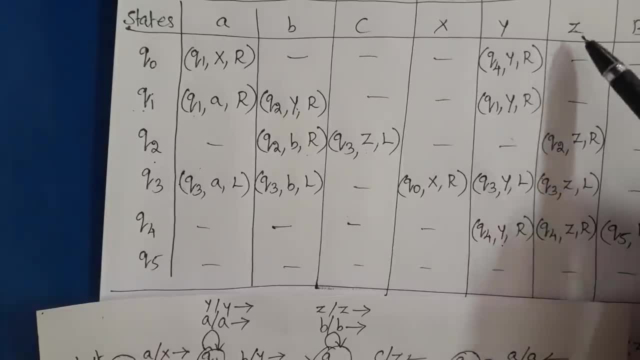 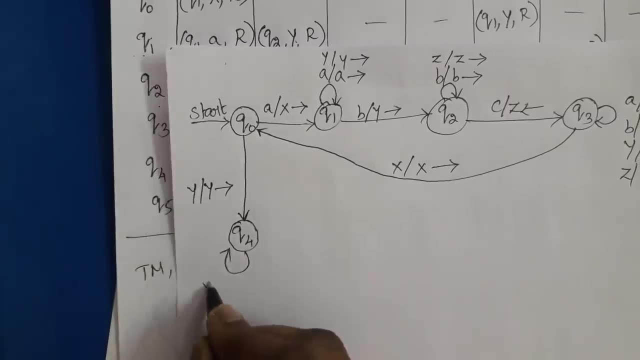 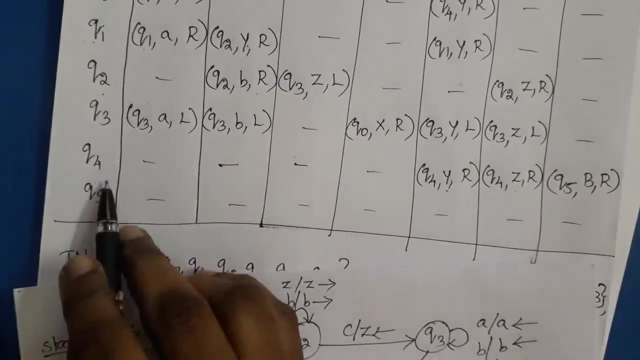 And from q4 to q4,. another transition is z slash z right move. So from q4 to q4, y slash y right move And z slash z right move. Then the final transition is q5 to blank.